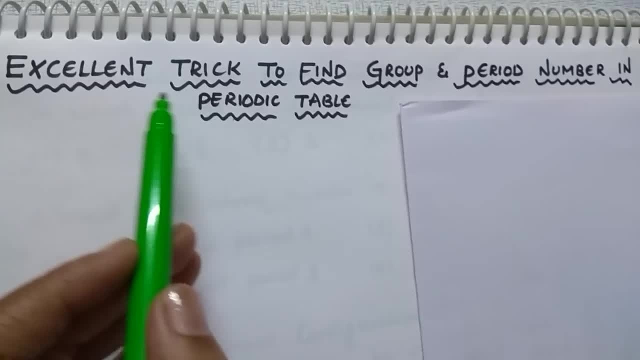 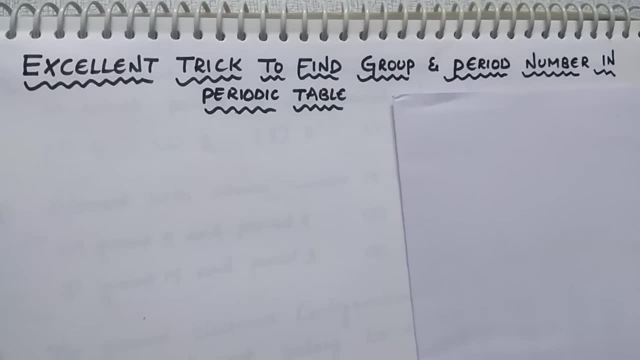 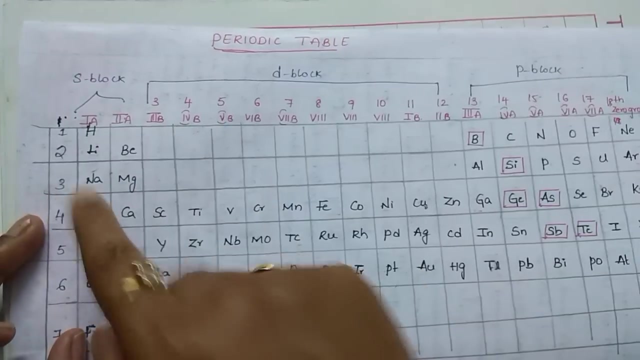 Hi students, in today's session I am going to discuss an excellent trick to find group number as well as period number in the periodic table. This is a modern periodic table given by Moseley, which consists of 7 periods. This horizontal row we call it as a period, like this: 7 periods are: 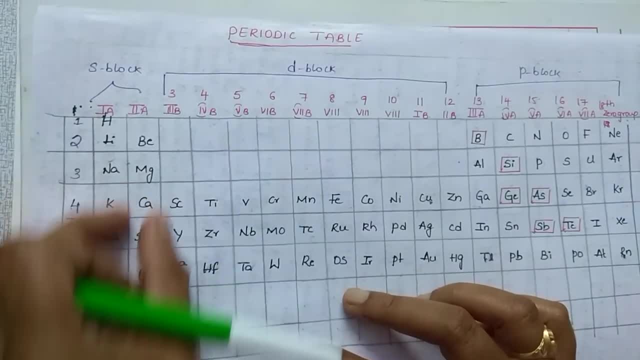 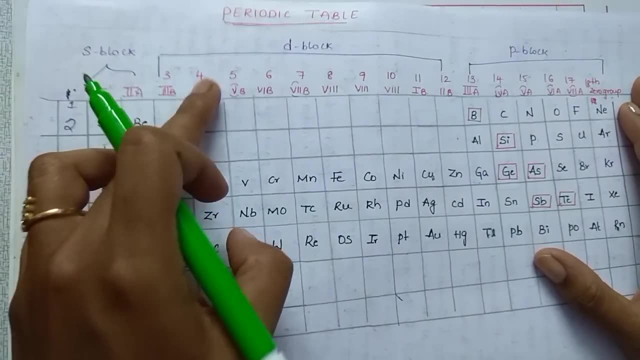 there and 18 vertical columns. This vertical column, this one, is named as a group. Total: 18 groups are there: 1,, 2,, 3,, 4, 5. up to 18 groups. How many periods students? 7 periods and 18 groups. 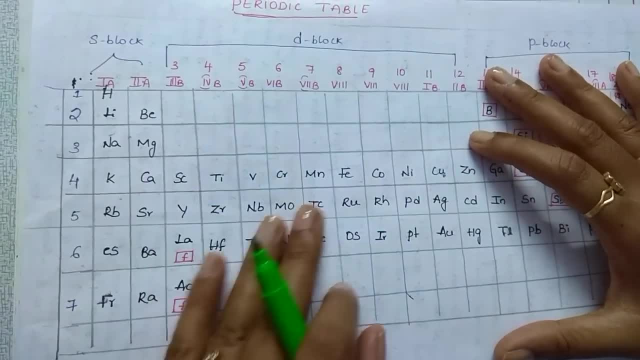 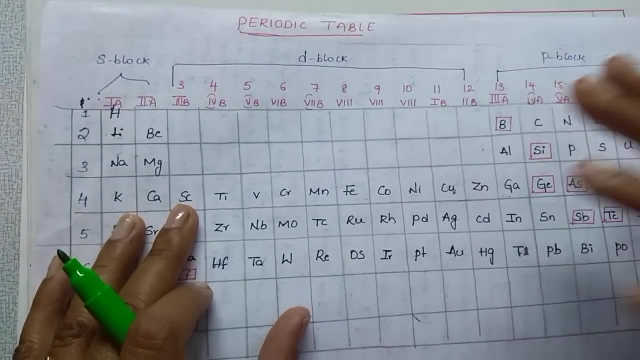 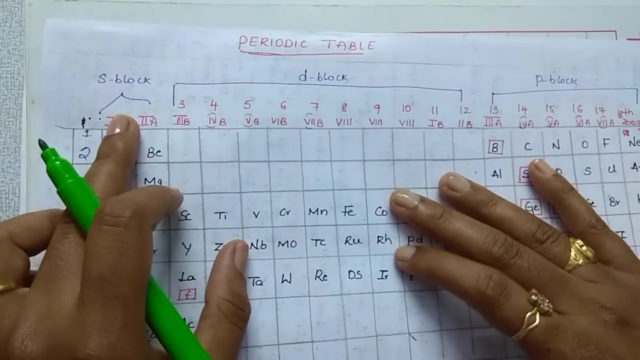 are there in the periodic table, and this periodic table is classified into 4 blocks: S, P, D, F. It is completely based upon last electron. If last electron- we say differentiation electron- If it enters into S subshell, then it is S block. If it enters into P subshell, P block. 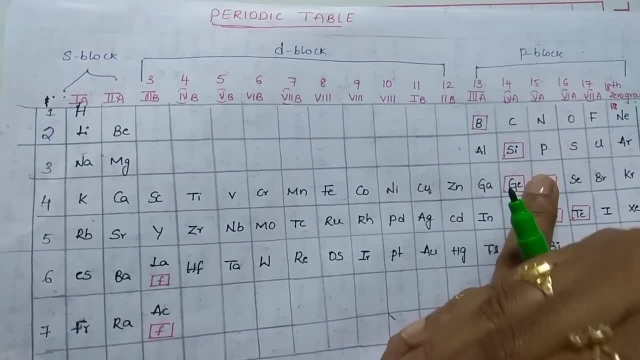 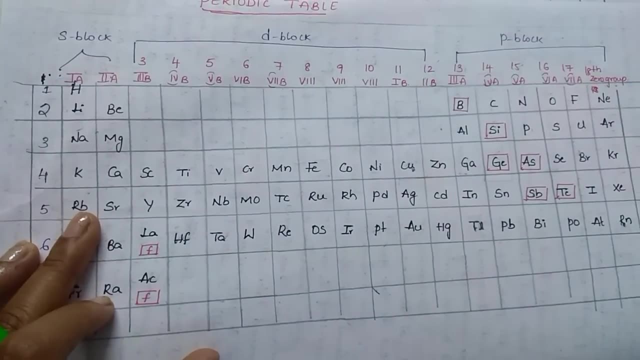 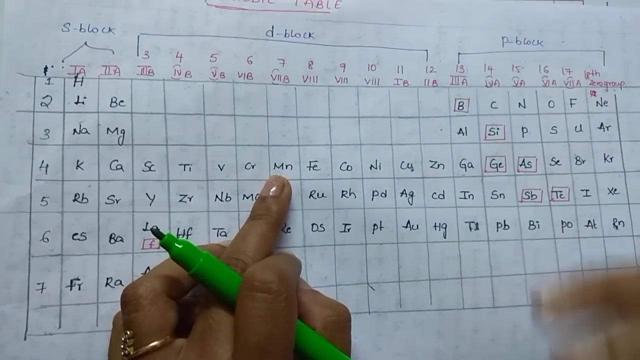 If it D, D block and F. If it enters into F subshell it is named as F block and those elements are called as F block elements. and suppose manganese is there. Manganese belongs to which group and which period in the periodic table? That is a question they ask in the exams. 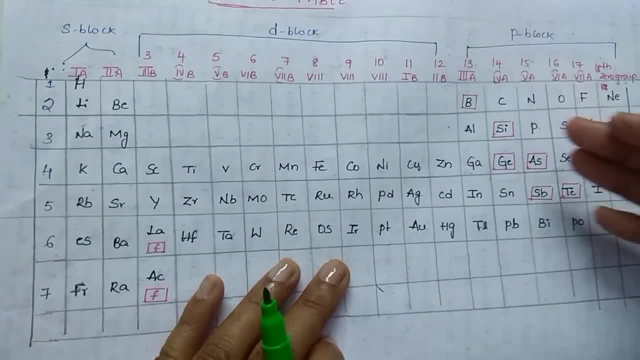 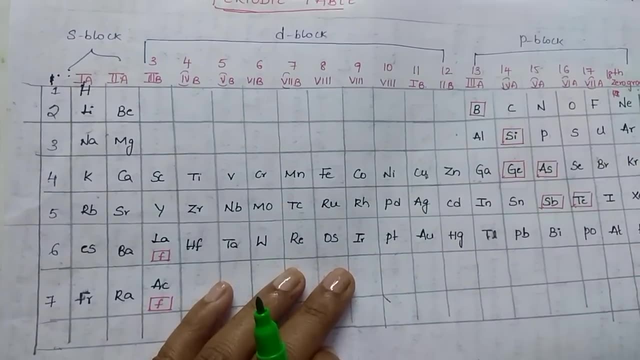 Strontium belongs to which group and period in the periodic table, Or nitrogen belongs to which group and which period in the periodic table. In today's session, I am going to tell you an excellent trick so that you can find the group number as well. 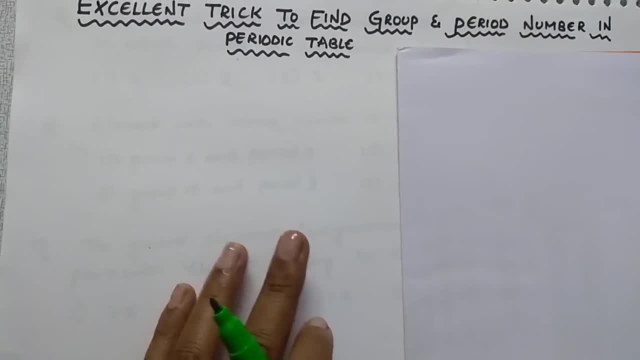 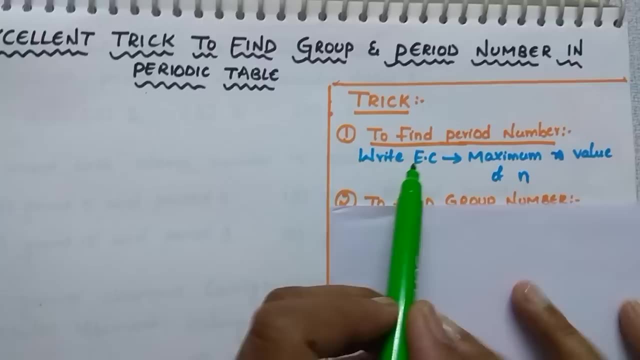 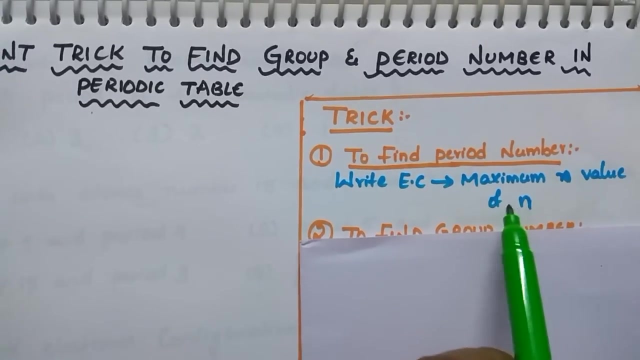 as a period number very easily. Let us start the trick To find the period number. the trick is: write the electronic configuration first. then, just after writing the electronic configuration, see the maximum number of periods. So let us start the trick. So let us start the trick. 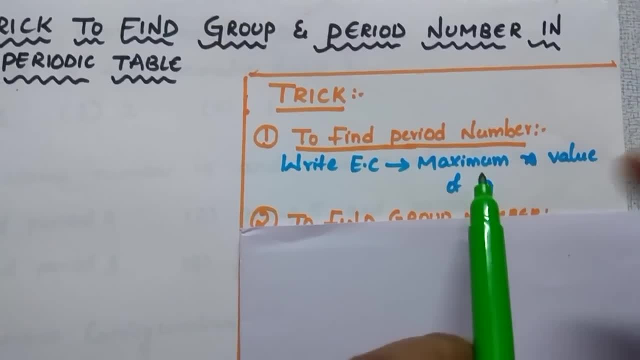 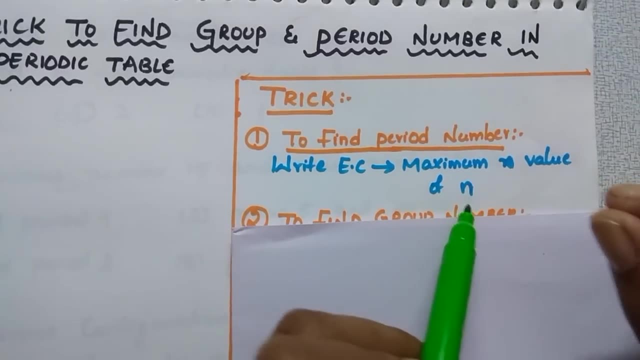 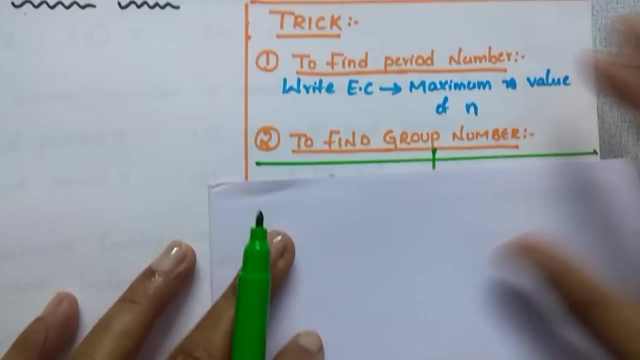 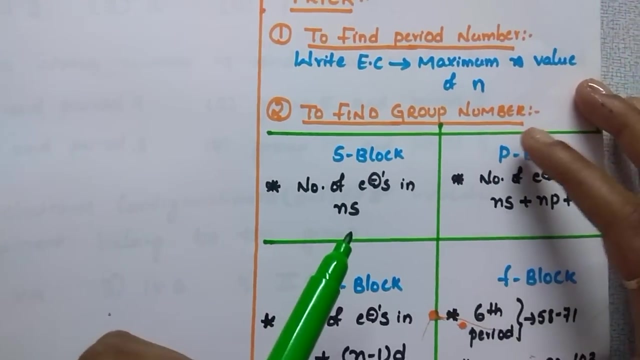 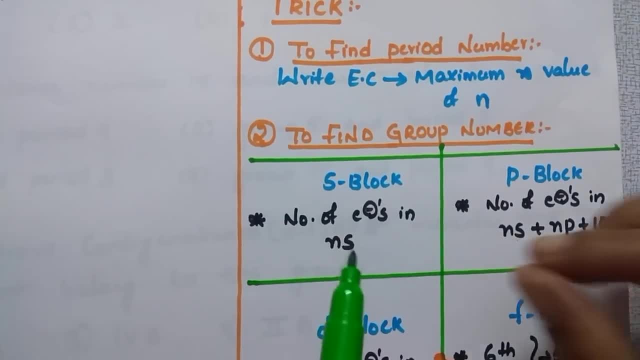 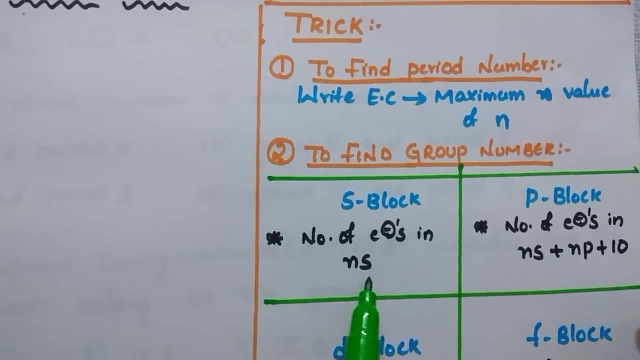 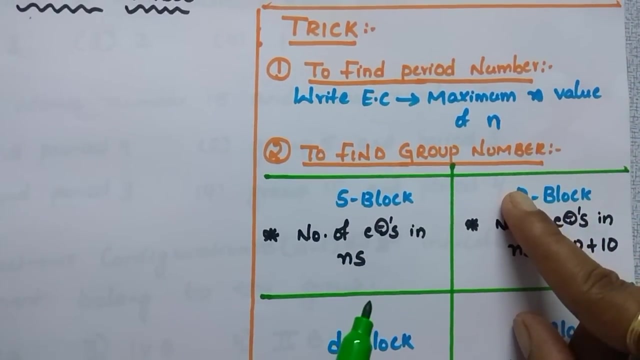 group: number of S block element. trick is just write the electronic configuration and count the number of electrons in ns. last electron enters into s subshell, then we call it as s block element. if, after writing the electronic configuration, suppose if the electron is there in the s subshell, then this trick you have to use. 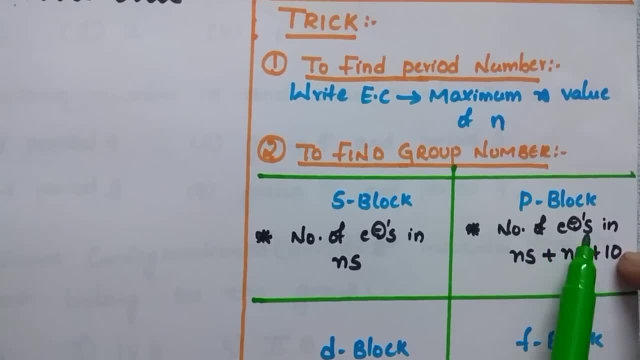 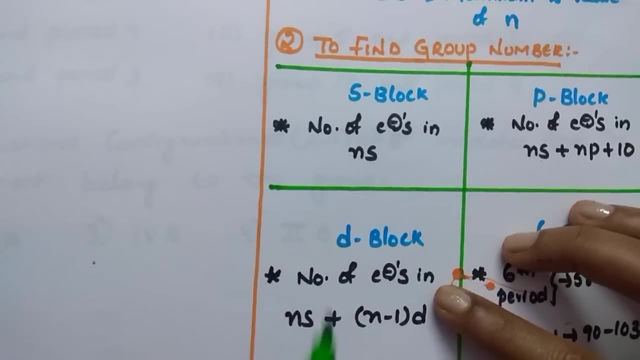 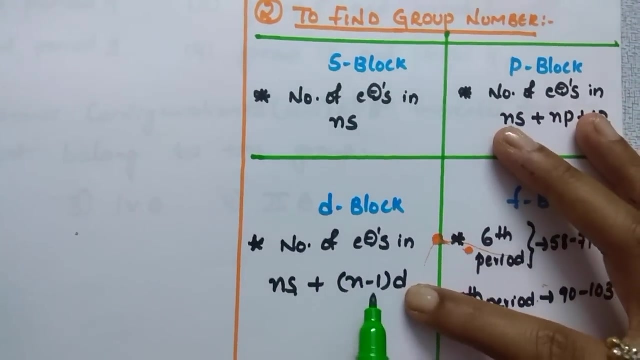 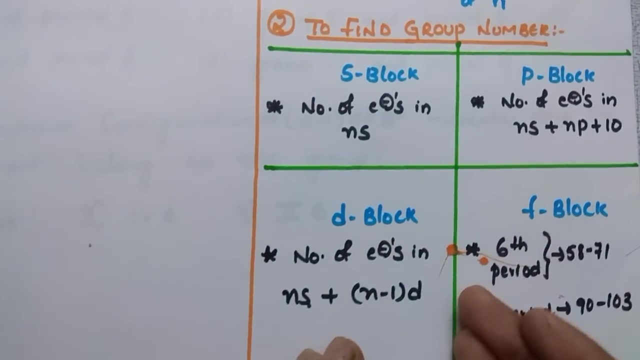 for the p block: number of electrons in ns plus np plus 10. this is the trick. for d block, the trick is write the electronic configuration count, the number of electrons in ns, as well as n minus 1, into d means the last shell and ultimate shell. penultimate shell, last shell before that shell. 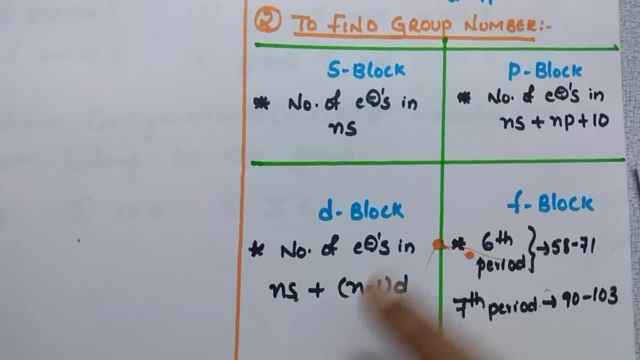 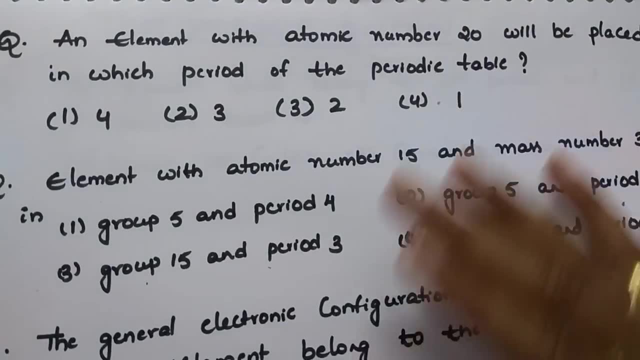 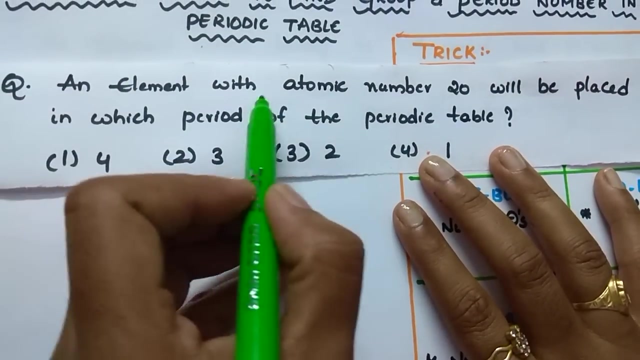 both the electrons, you have to count for d. that gives the group number. so let us see few questions. by using these tricks you can solve these questions very easily. let us see this question. an element with atomic number 20 will be placed in which period of the? 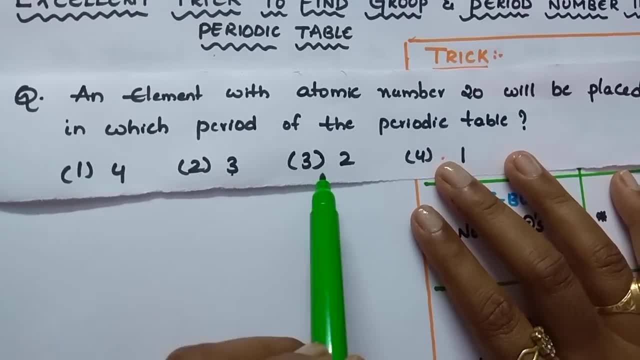 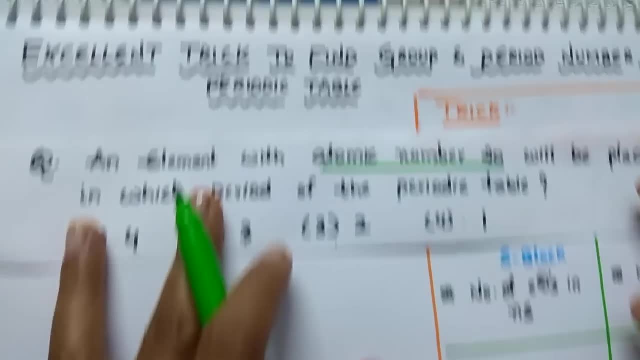 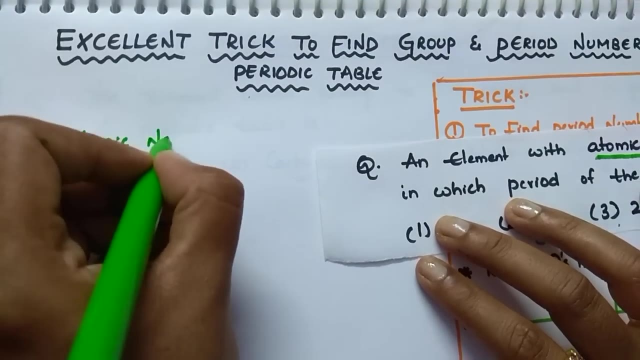 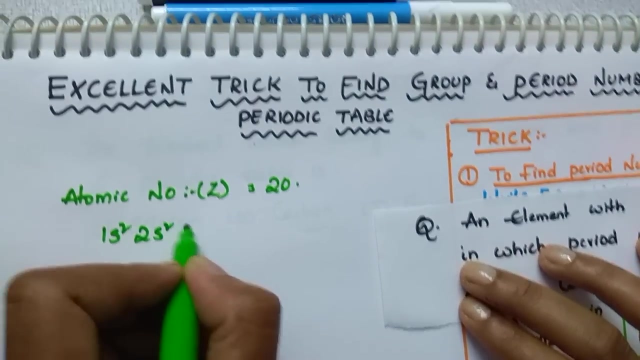 periodic table: 4, 3, 2, 1. what is the atomic number? student atomic number 20. so what is the trick? first write the electronic configuration. atomic number 20. electronic configuration: 1 s 2, 2 s 2. see, you should know, you should have an idea of writing. 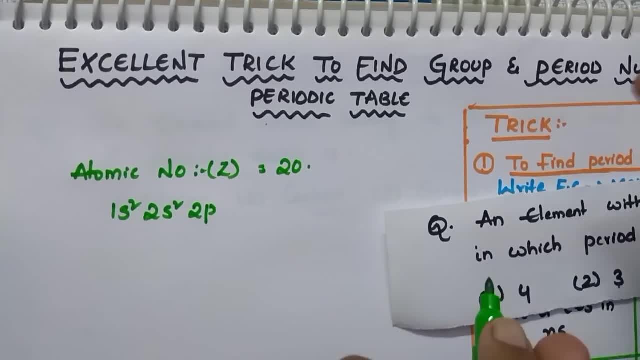 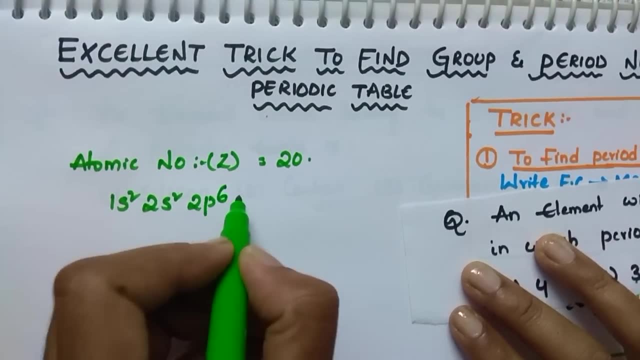 the electronic configuration, suppose if you dont know. means learn and use this trick without knowing electronic configuration. you cannot find 2, p, 6, 3 s 2, 3, p, 6, 4, s, 2. everyday is earth here very peaceful, doing thelectronic. 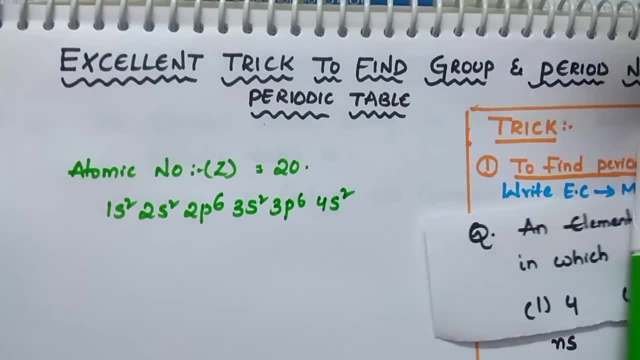 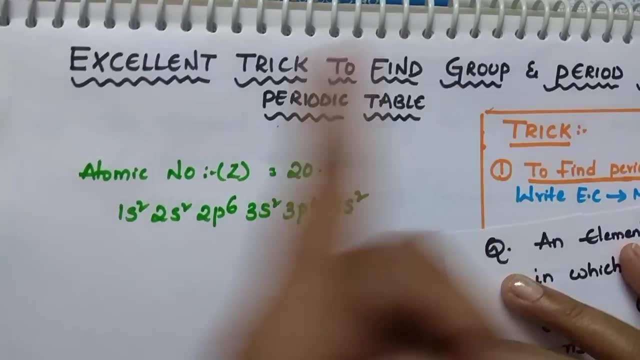 ok, lets run it. the electric선p yawr email jw latous' etw propre pickles is the electronic configuration, and last electron enters into which sub shell s sub shell, so this one, this element belongs to which block s block element? in the case of s block element, what is? 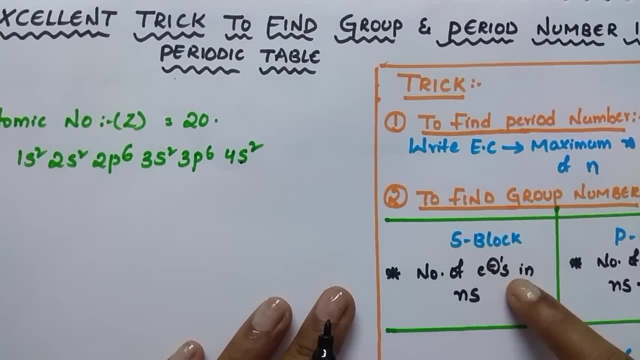 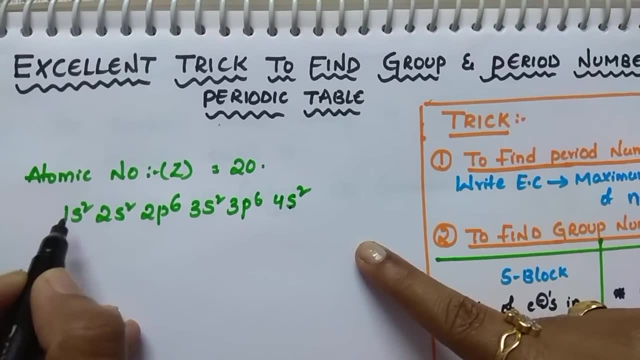 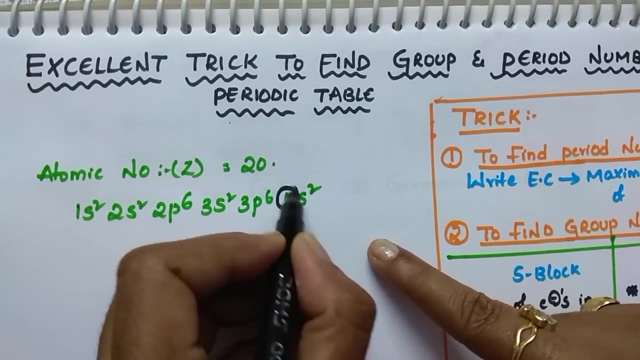 the trick to find the group number: just count the number of electrons in n s last shell. what is the last shell here? actually? n value. see here n value is one principal quantum number, here two, three, four. maximum n value is four. maximum value of n gives which one period number, so here maximum. 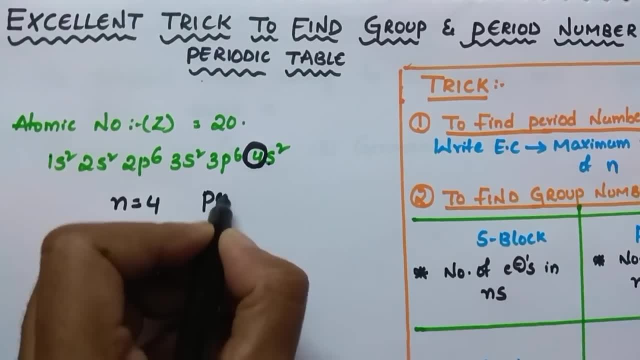 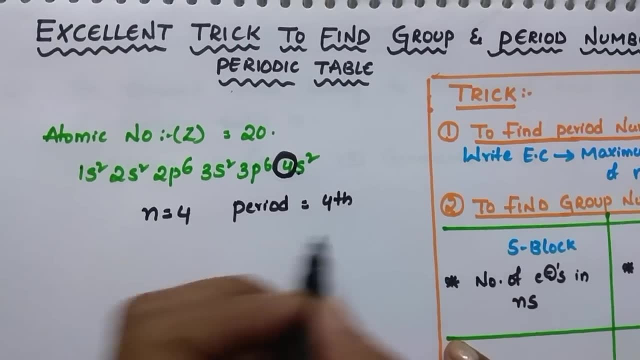 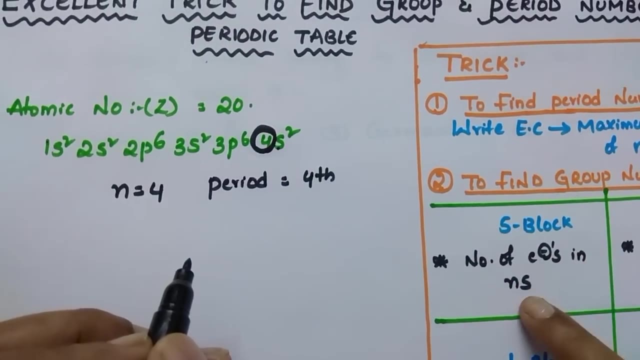 n value is four. so period, which period it belongs to. fourth period period. fourth, coming to the group number, the, it belongs to s block. this element belongs to s block. so number of electrons in n s last s, last shell 4s. how many electrons before grupo Vlad? What is the period of n 항? where? period of s which belongs to group? 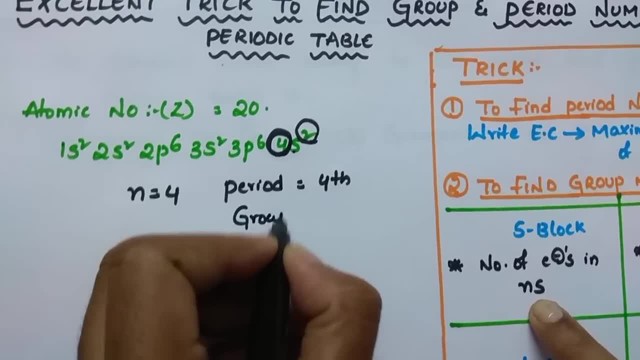 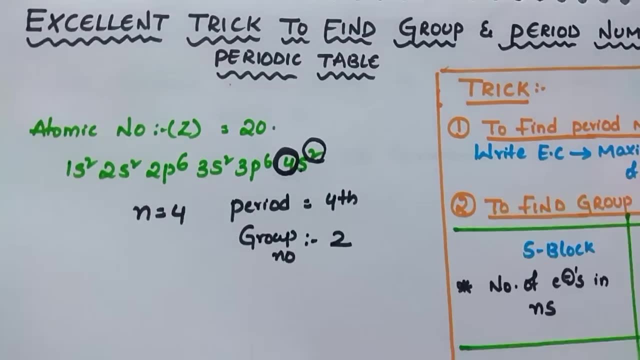 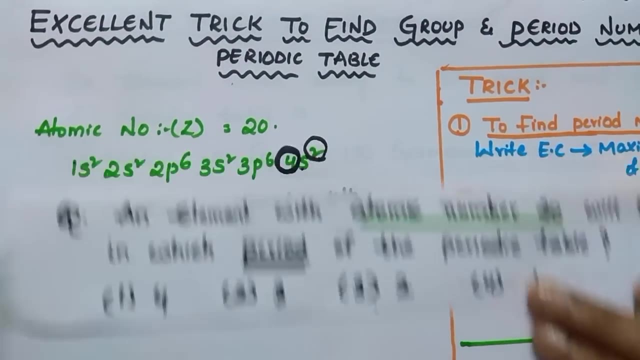 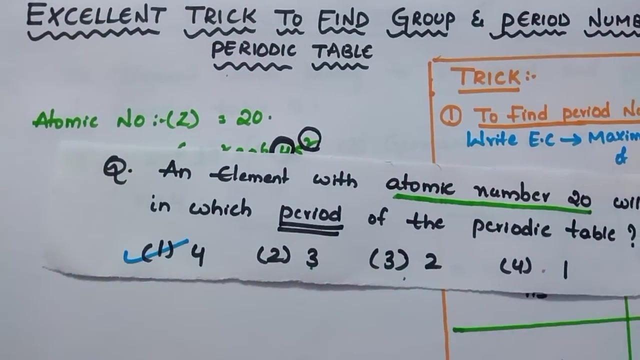 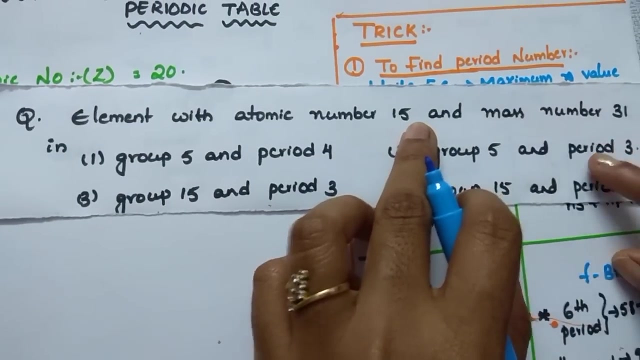 are there students? 2 electrons, So group number is 2.. Then what is our answer? They are asking: which period Period is which one 4th period? This is your answer. Let us see one more question. Element with atomic number 15 and mass number 31 is present, in which 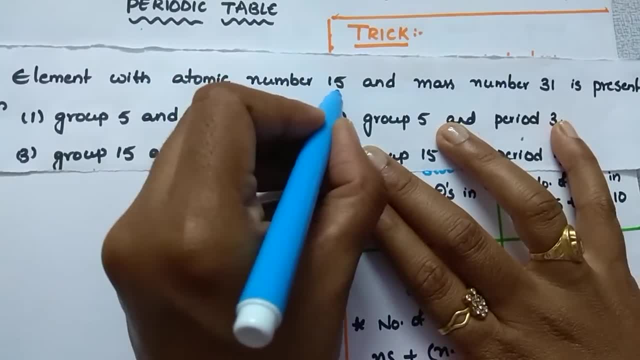 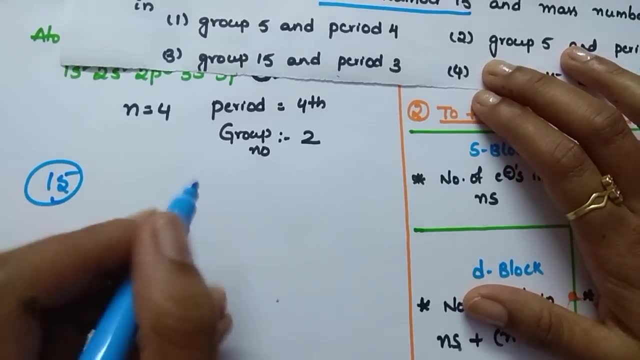 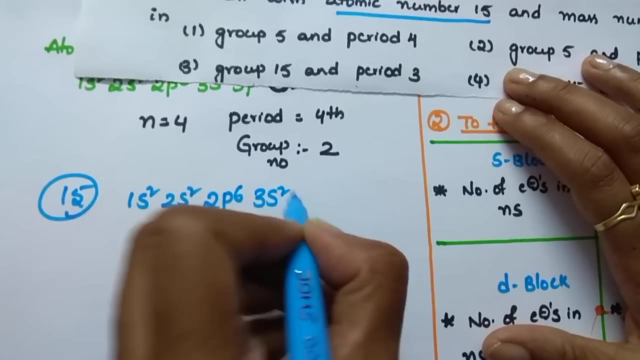 group and which period you have to find. What is the atomic number? student 51.. If atomic number is 15, then what is the electronic configuration? 1s2, 2s2, 2p6, 3s2, 3p3.. What is the atomic? 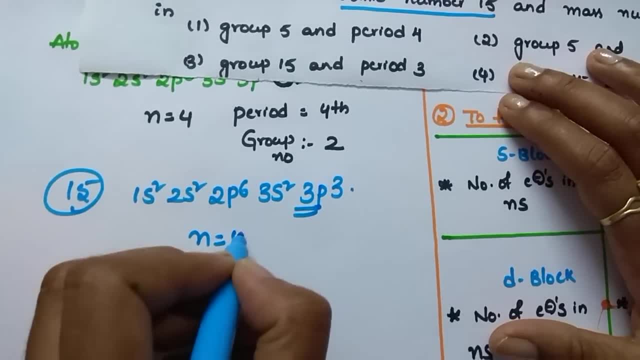 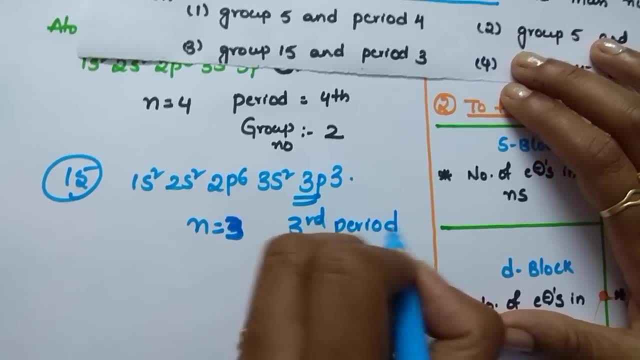 number 1s2,, 2p6,, 3p3.. What is the maximum value of n? 3.. n is equal to 3.. What is the period number- 3rd period- It belongs to 3rd period And what is the group number To find? 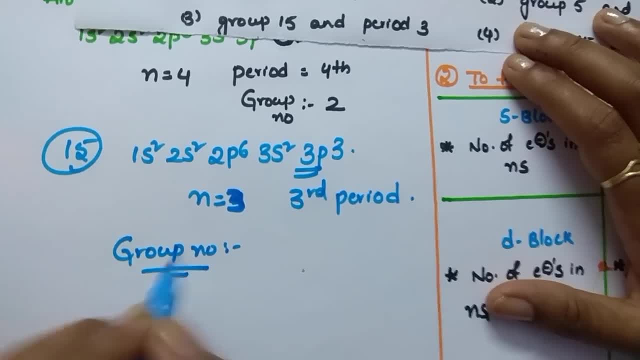 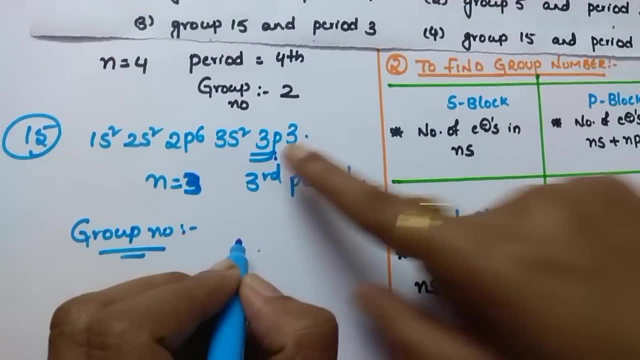 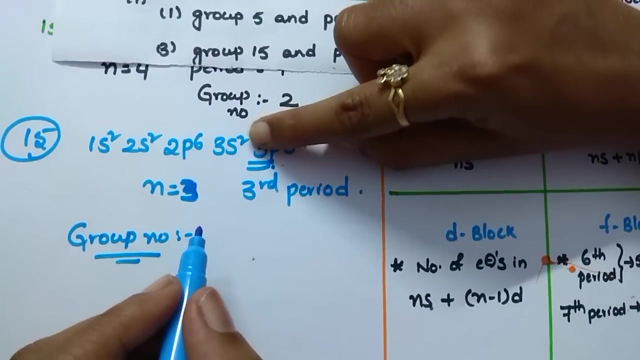 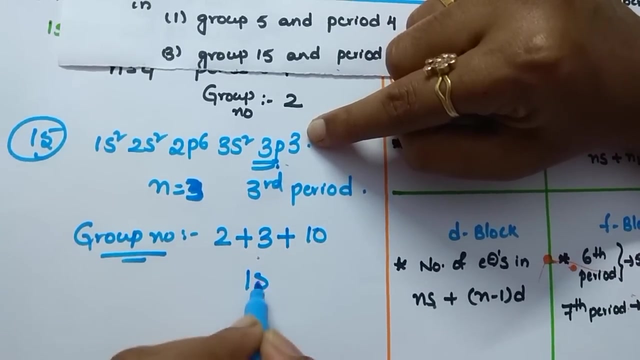 the group number what you should do First. you should see this particular element belongs to which block. Last electron enters into the p. so it belongs to p block, P block. what is the trick? Number of electrons: s plus p plus 10.. Ns has how many electrons This? 2 plus p has how many electrons 3 plus 10.. So belongs: 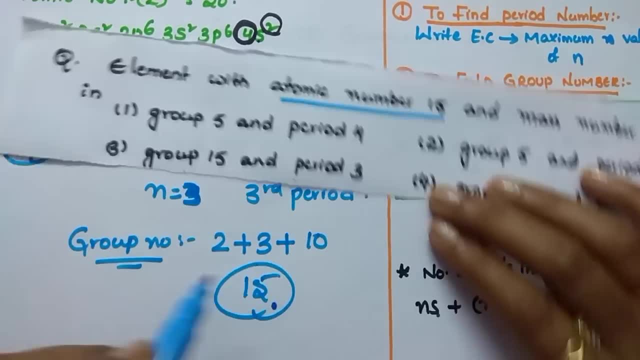 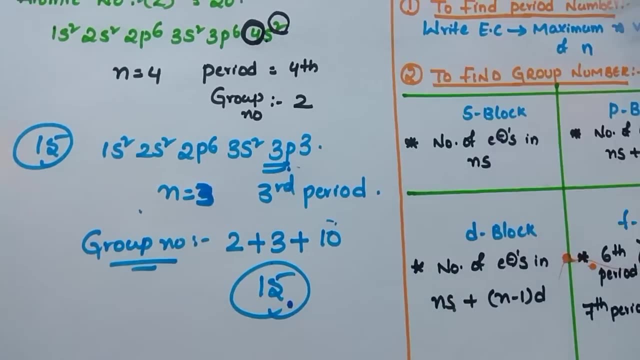 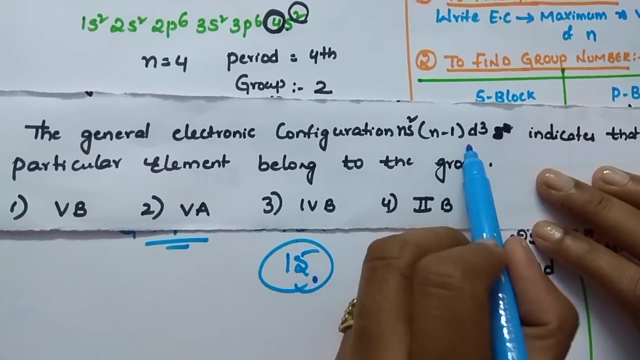 to this. one belongs to 15th group, 15th group and 3rd period. This is your answer. Let us see one more question. The general electronic configuration of an element is ns2- n-1d3.. Now you have to find the group number Ns2- n-1d3.. Now you have to find the group number Ns2. 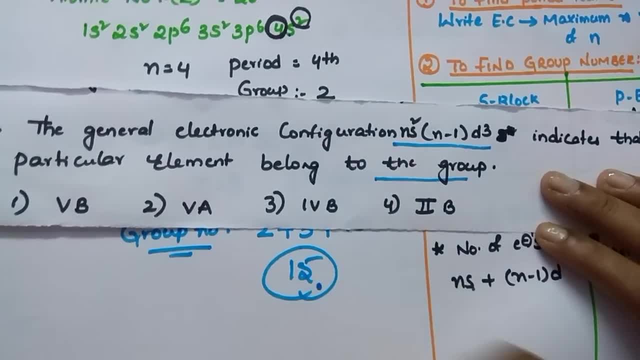 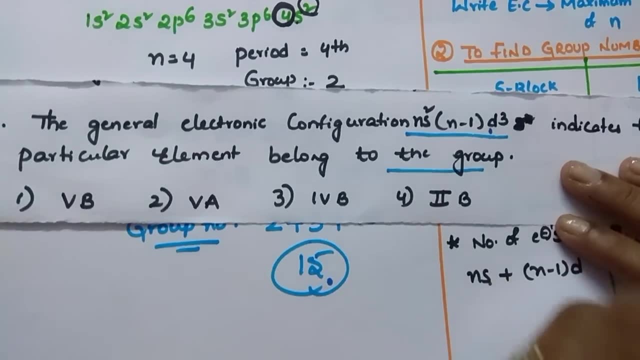 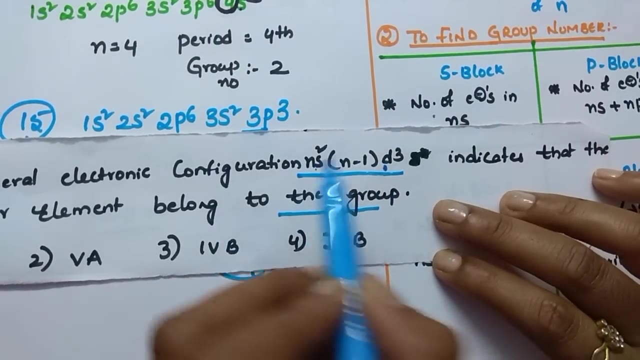 n-1d3.. Now you have to find this particular element belongs to which group in the periodic table. Last electron enters into the d. So it belongs to which element, students? It belongs to d block. What is the trick? Ns electrons plus n-1d electrons. Ns electrons- how many? 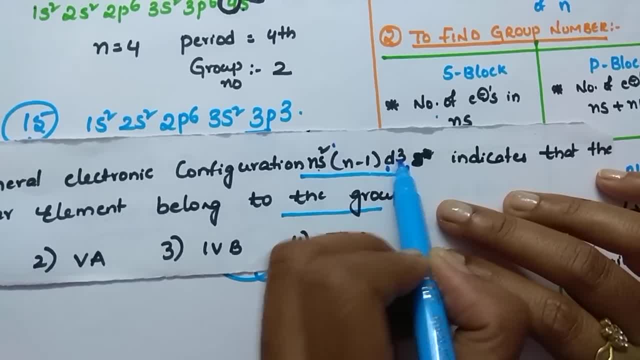 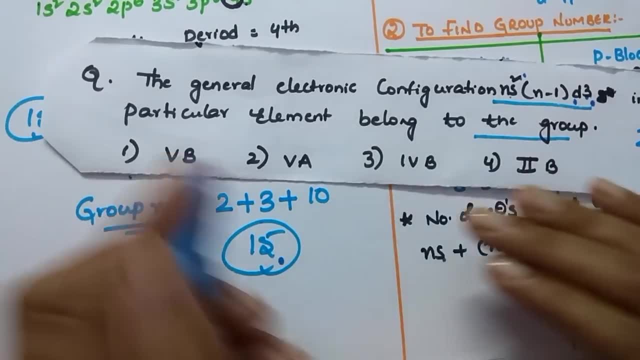 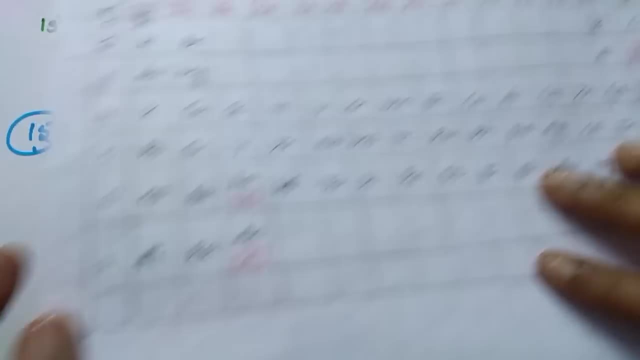 2 and n-1d electrons is 3.. 2 plus 3. Total. it belongs to which group- 5th group, In this case 50a- is given, Which is what is the answer? 5th b is the answer. Why, See, this is the. 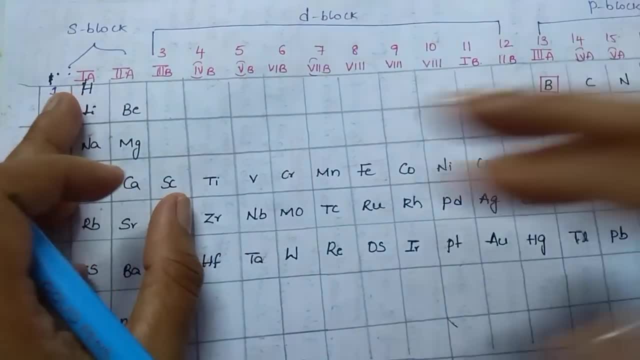 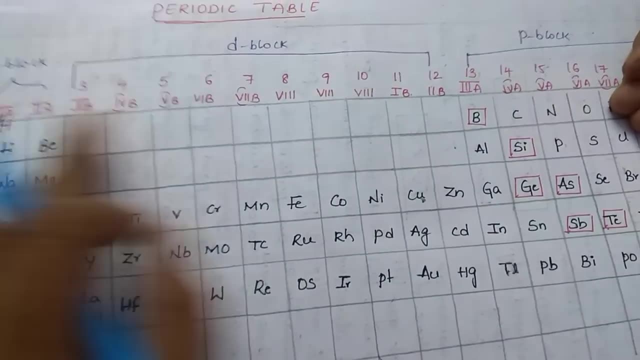 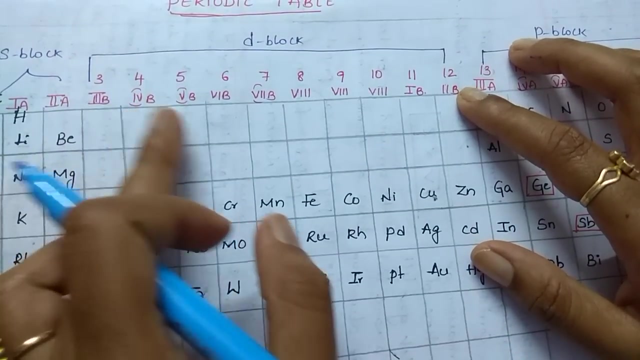 periodic table which is named as 1,, 2,, 3 and in that 1a, 2a s block, 3a, 4a, 5a, 6a. these are p block and d block starts from 1b, 2b, 3b, 4b, 5b. d block comes under 3b, 4b, 5b. 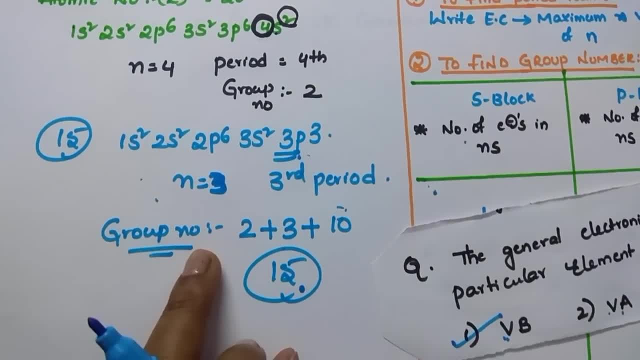 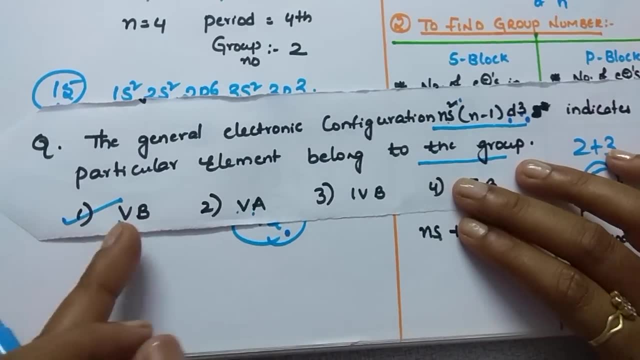 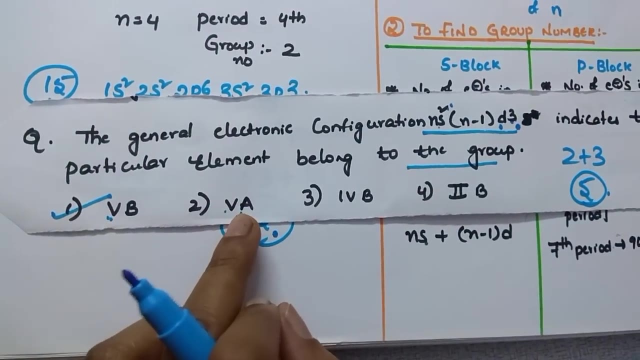 right. This element comes under which block This element comes under which block This element comes under? So 5b comes under b, comes under d, a comes under either 1a, 2a or s block, and 3a up to 8a comes under p block. Okay, And let us see the test yourself. question. 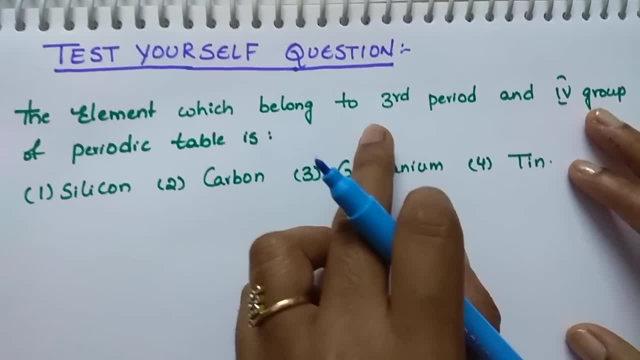 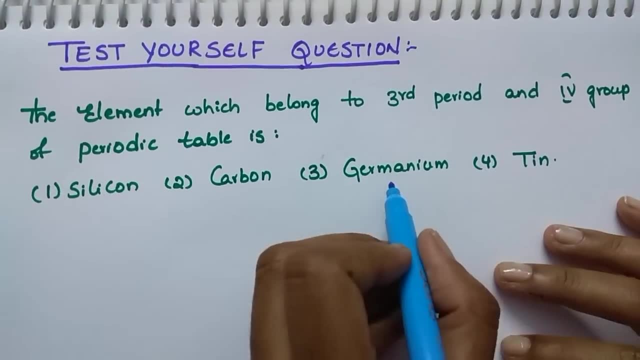 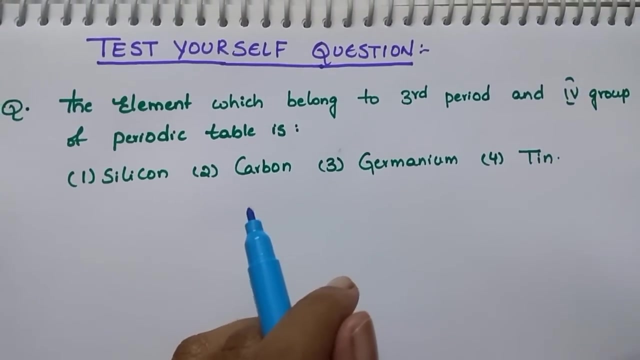 as your favorite. The element which belongs to 3rd period and 4th group of periodic table is Silicon Carbon Germanium Tin. Just use this trick and find out which element it belongs to. First write the electronic configuration and then find out. I am going. 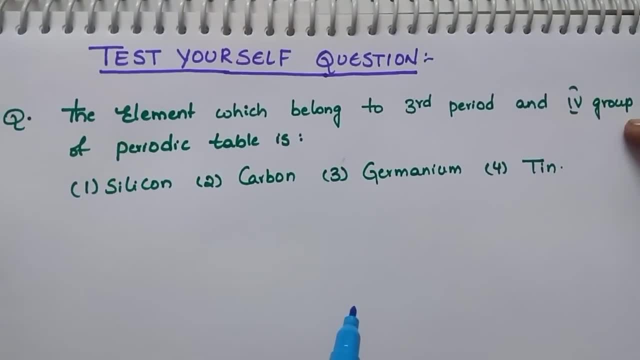 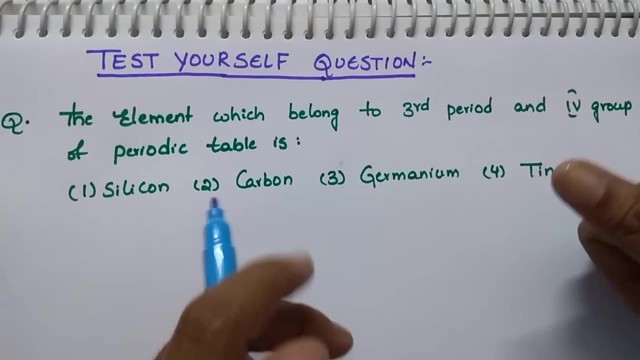 to give the solution to this one in the description box. Don't see the answer directly. First try it and then go through the solution link. If you get the right answer, please click on like and comment me that you got the right answer. One more thing I forgot to tell you. 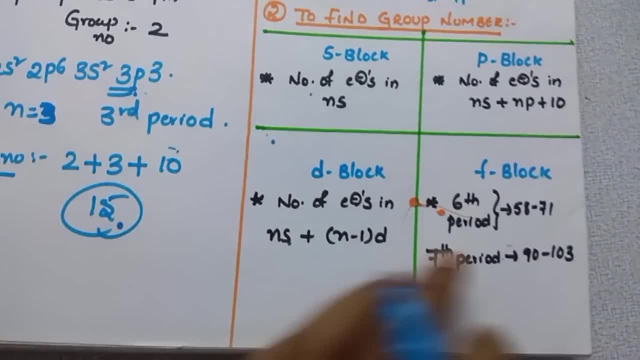 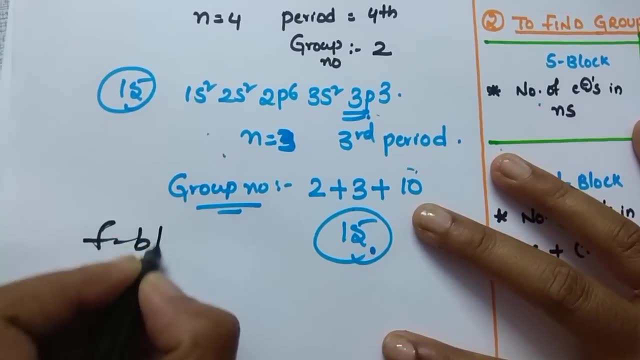 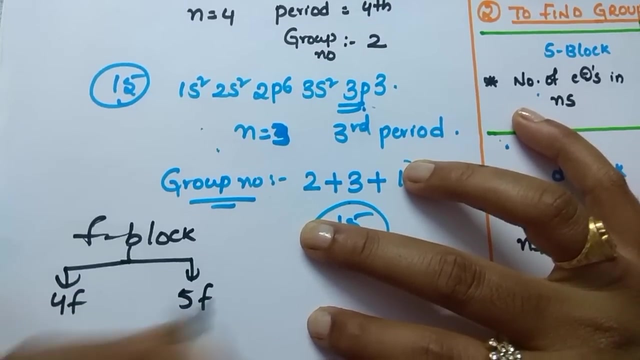 Coming to the f block, f block. if you see, here it consists of f block elements 2 series. f block 2 series. f block 2 series. One is 4f, other one is 5f. Lanthanides- actinides- Lanthanide element. 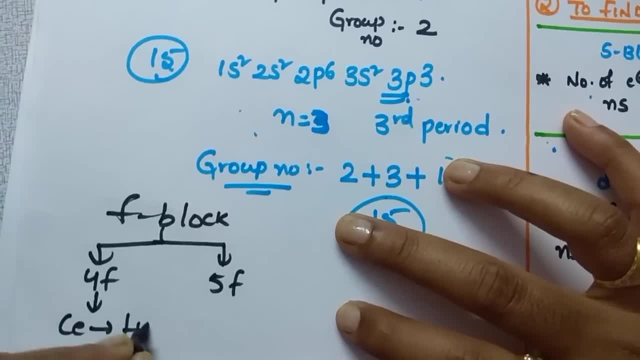 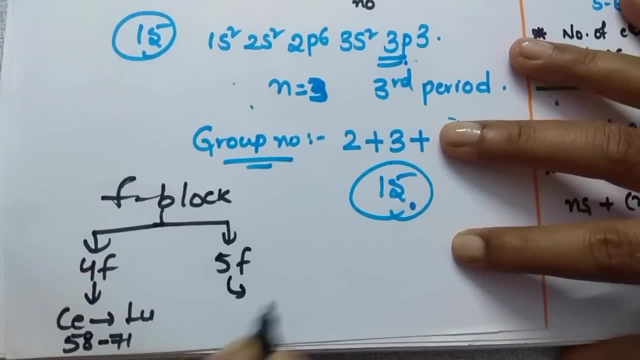 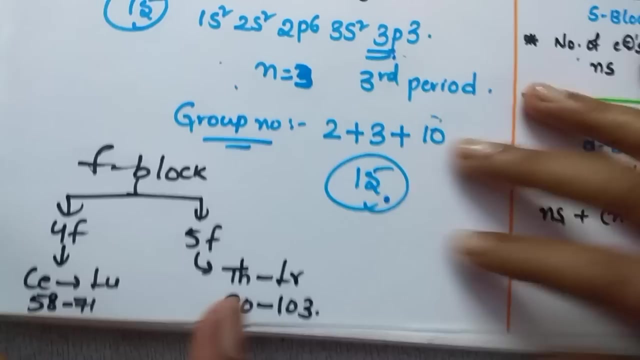 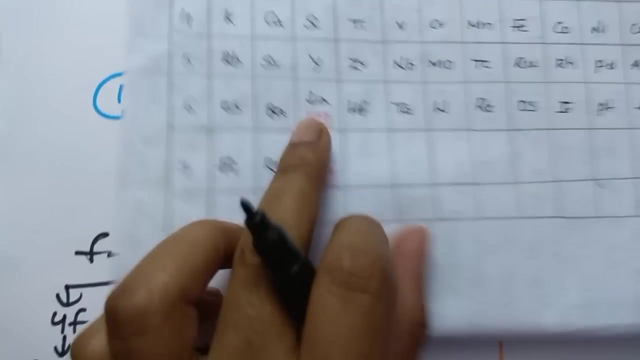 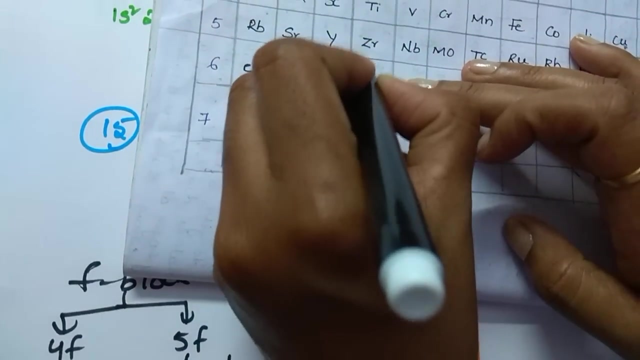 starts from cerium to lutetium, of atomic number 58 to 71, and 5f series actinides starts from thorium to laurentium, atomic number 90 to 103.. Okay, This is a normal thing. If you want to see this, maximum problems, log under last. 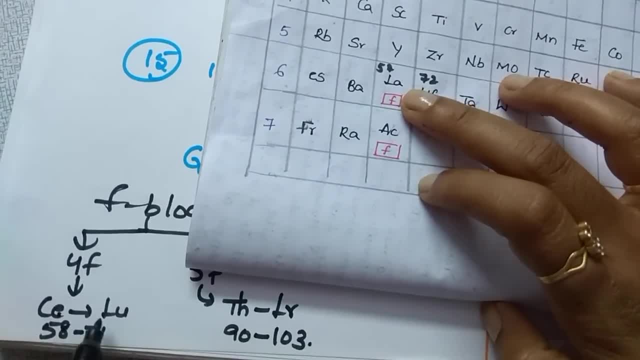 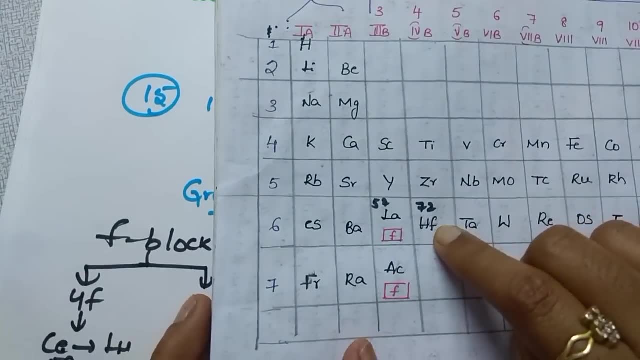 is. So everything looks like this, So Let's see the periodic table once. this is the periodic table. Lanthanium atomic number is 57.. Laurentium atomic number is 72.. After this lanthanum element cerium starts up to. 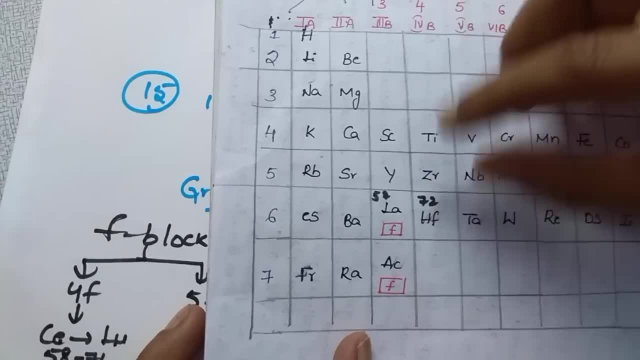 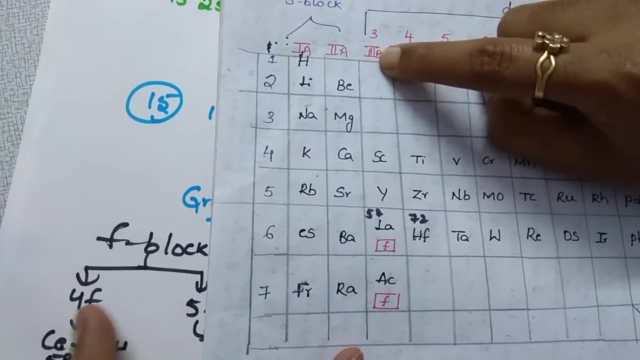 Lutetium means before H, integrated with sequel atom's, and these elements comes between lanthanum. these two elements, this group comes, so it comes under which one third b group it comes under after lanthanum. that is the reason these elements, f block elements, comes under third b for actinides. 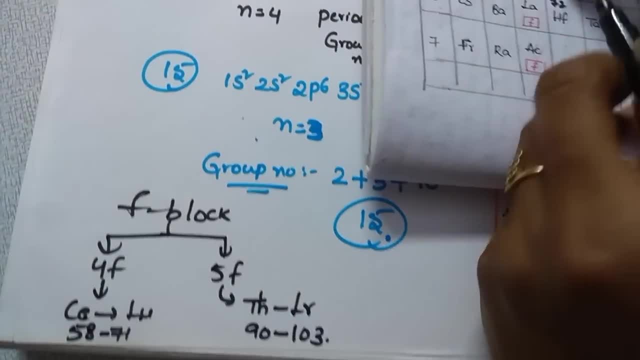 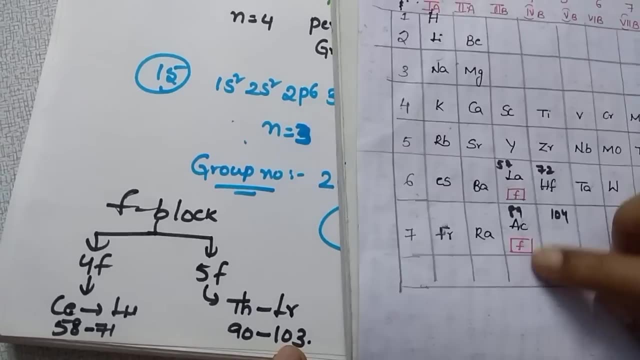 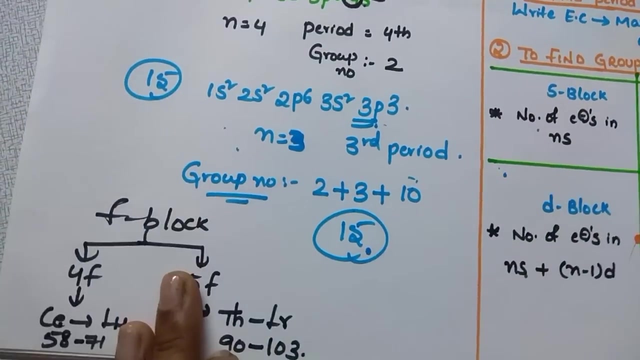 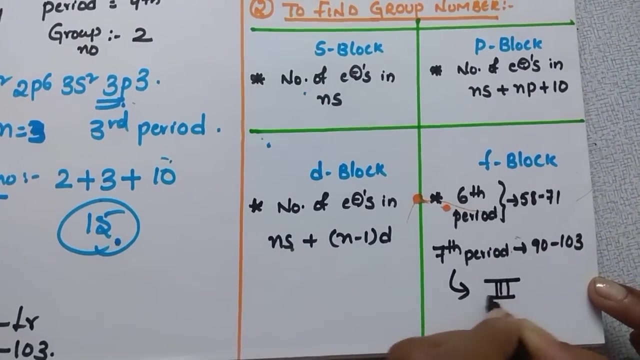 also same way, thor. actinium atomic number is 89 and next element atomic number is 104. this actinide series 92, 103 comes under after actinium. means here same group. it falls third b. so whenever they ask the elements of f block, the trick is just they belongs to third b or third group. third group.